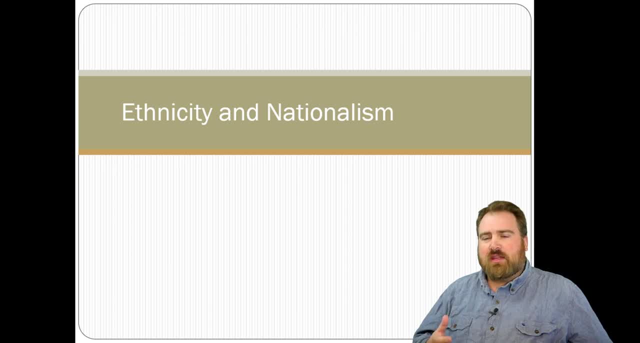 whatever subject that you're looking into, and pick something within that subject, Maybe find a couple of specific things that you're interested in finding out about. When we're doing anthropology, we take this approach of the holistic approach. We want to hear about everything and see about. 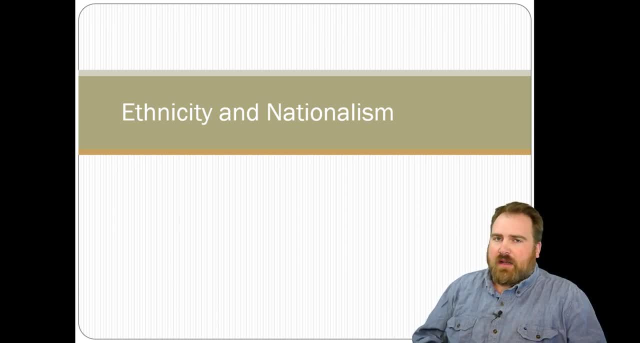 everything and include everything. We also have to recognize that there are limitations and that for a five-page paper, you just can't get everything in it And not have anything. that's really serious. So what I'd like you to do is: whatever. subject. 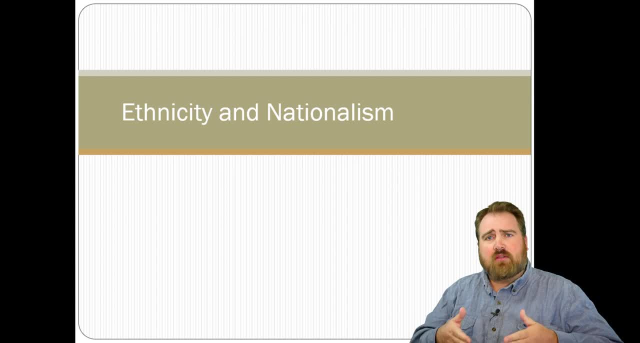 that you end up choosing. you know, narrow it down a little bit, Come up with some specific questions that you want to ask and then kind of focus on those questions, whatever that subject is. The other thing that's been brought up is that you need to have two interview. 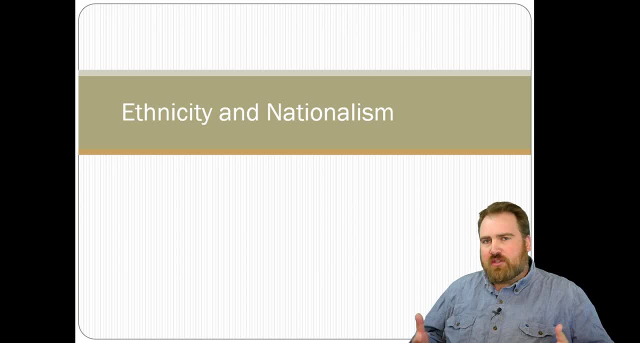 interviewees, Two people that you're going to interview about your subject, Two- And you're going to be interviewing them in two different ways. You're going to be doing sort of a- Oh my goodness, I just totally forgot what they're called. You're going to have a structured interview and you're going to have an informal. 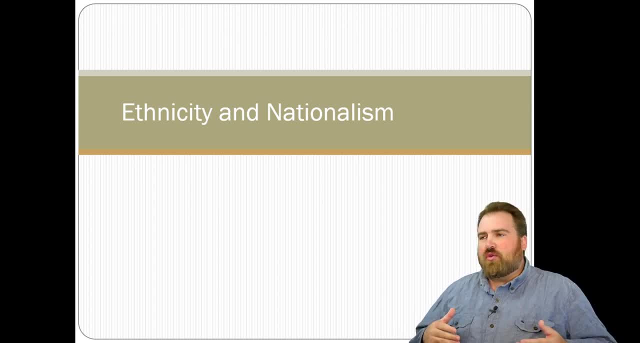 interview. okay. so the structured interview is where you basically create a series of questions that you're gonna ask both of your participants, and if you want to add in more participants, that's okay too, but the minimum is two, so that you need to have a series of structured questions that you ask each of your participants. 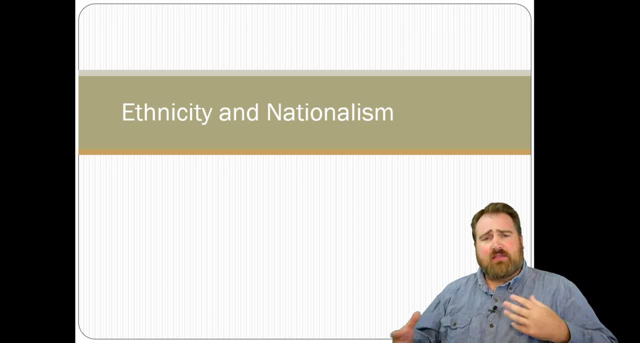 and this is to give you a baseline set of information. like: this person says this, this person says that, right, so you can, you can address each one and see how they correlate, how they differ. and then there's the, the unstructured interview, the, the, the casual interview, in which essentially, what you're doing is you're. 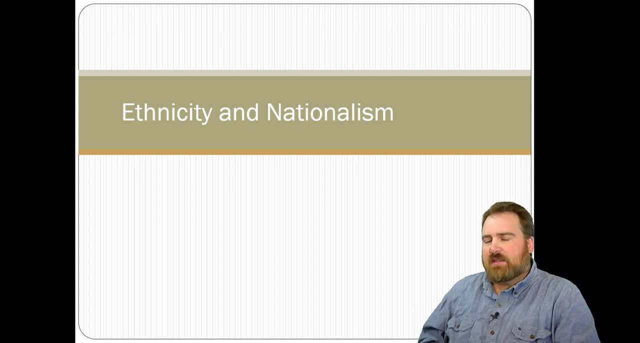 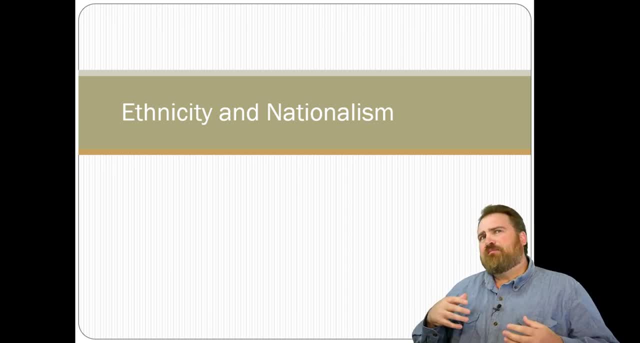 you come up and say, okay, well, you know, I have this question, and and your person starts answering that question, and then, as you're listening, all of a sudden a new question pops into your head and you're like, oh, I should ask about that. and so then you ask about that. and then that goes to another question and it's: 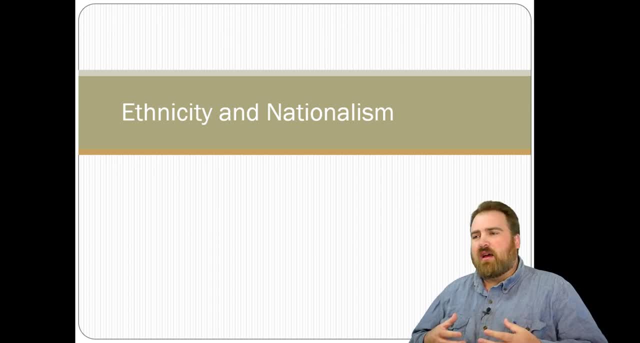 kind of freeform. it's a freeform interview basically, so it's not necessarily structured. you might have a few questions that you start out with, but you really kind of want your people to answer and ramble right and just come up with whatever information they come up with, let them sort of dictate the. 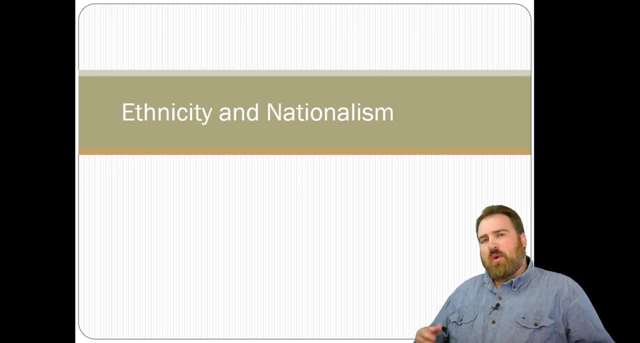 information that that they're giving you, and then have questions set aside so you know if you cover a subject and that person is done, then you know you can go on to the next person or to the next question and ask those questions. so these unstructured interviews are a lot easier to understand and you can kind of just 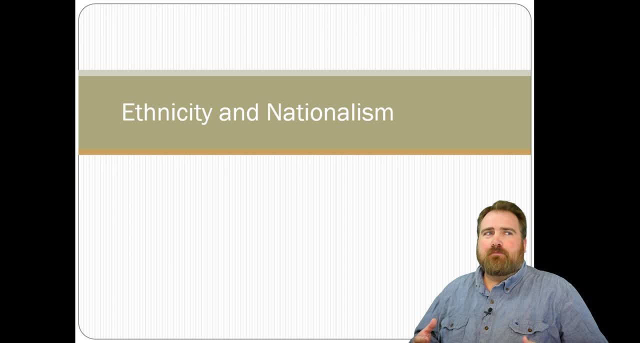 go through all of the questions. you need to understand and kind of figure out what they're asking for. to get to the next person, you're going to have a good overview of what they're asking you to do in your interview and if you are doing a few interviews, you might have the same basic set of questions as you're. 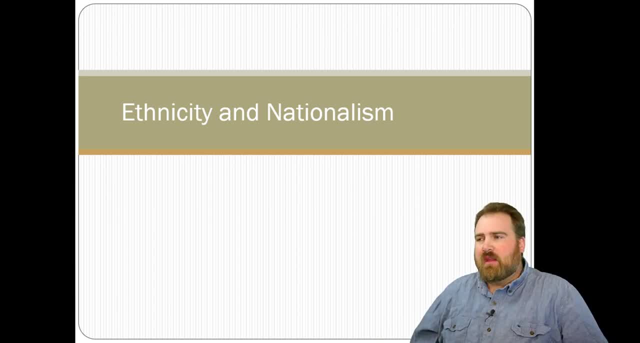 going to ask each person, but they do not have to turn out in the same way. you don't have to ask the same questions to each one, which is why it's informal. so you've got those two different types of questions that you need to answer, or two. 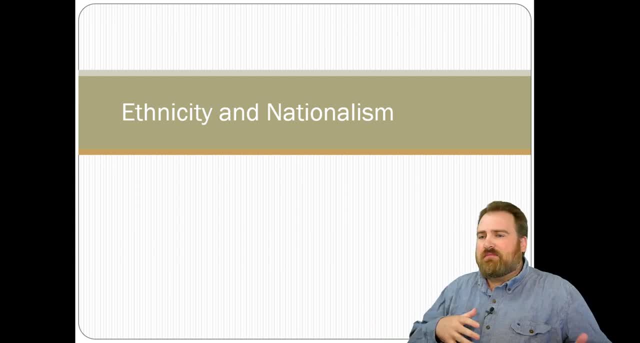 informal, And so, basically, you know, figure out, you know what your subject is and then start thinking about those questions like creating a battery of questions, And those questions should sort of be structured around the four subjects that I want you to take into consideration. 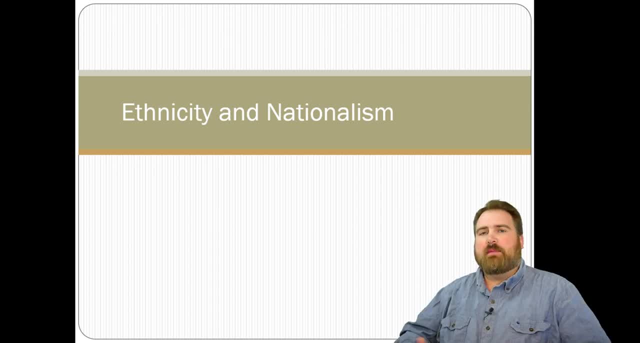 as you're developing these questions right. So those four subjects could be, say, you know, language, religion, race and gender, right, Those four things could be sort of the focus of some of your questions, or at least you know will somehow incorporate those four things into. 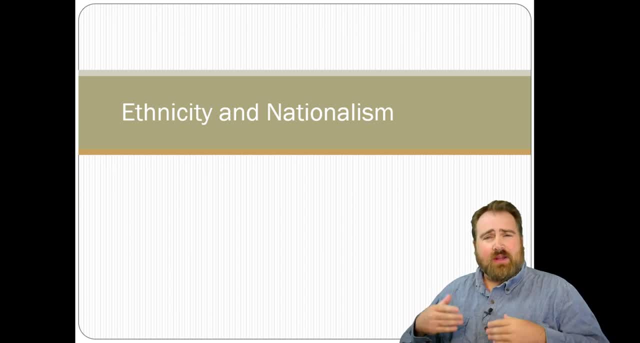 your battery of questions that you end up asking. So you want to incorporate something like that. It doesn't have to be those four, you know. if you want to incorporate one that talks about the norms of a community, If you want to talk, if you want. 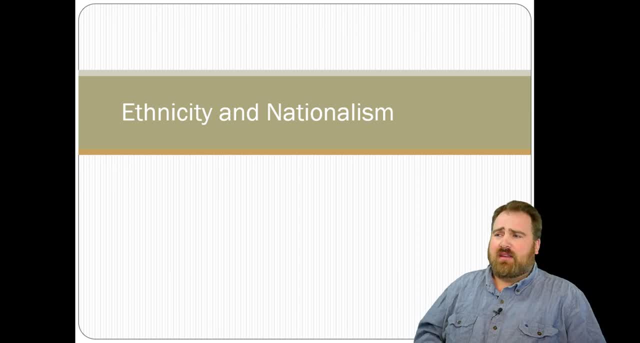 to bring in. you know, gender and sexuality, combined with race and inequality. those are four subjects that you can, you know, toss in. So there's, you know. you can take anything that we're going to be covering throughout the semester and create your own combination of. 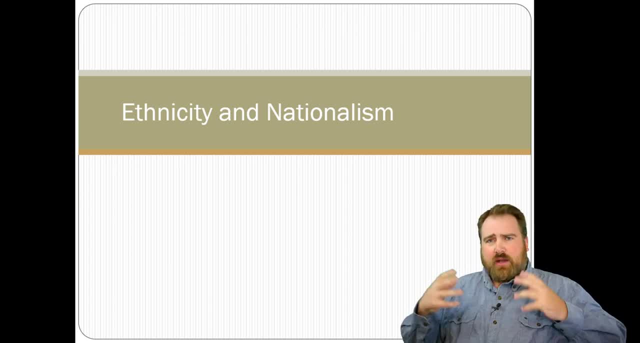 four subjects that you can, you know, toss in. So there's, you know you can take anything that you want to incorporate into this paper, okay, So, but those four things are totally up to you. So, yeah, the thing that you need to come away from this is is that if you haven't emailed me, 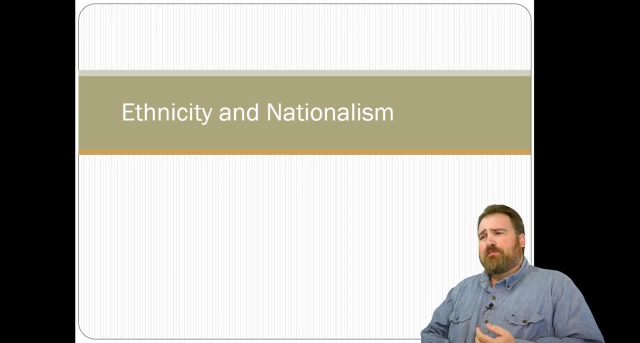 what your subject is. do so And then it's so that I know what you're doing and that if there's any questions or concerns, I can bring them up. That there are two types of subjects that you can incorporate into this paper. 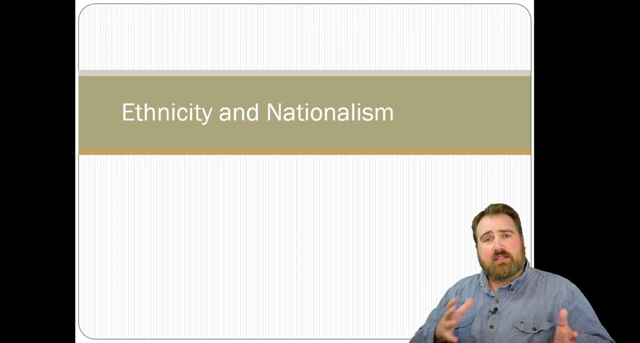 So there's the. you know you have to have two participants, right, You have to have two people that you can interview. You're going to do two different types of interviews with those two people: the structured interview and the informal interview. And then, you know, pick your four. 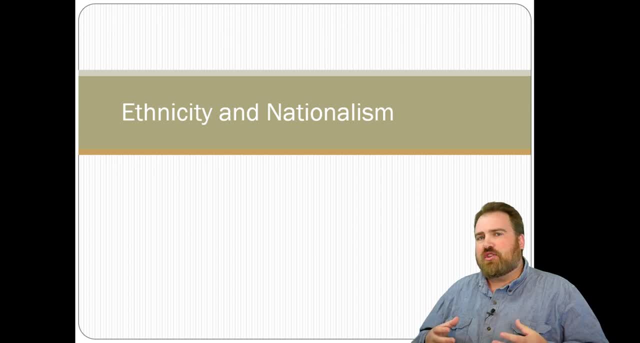 subjects. right, Pick the four subjects that you're going to choose to use. So yeah, So if you haven't got that to me, go ahead and do it. I'll see you at the workshop. Thank you so much. See you in the next one. Bye. 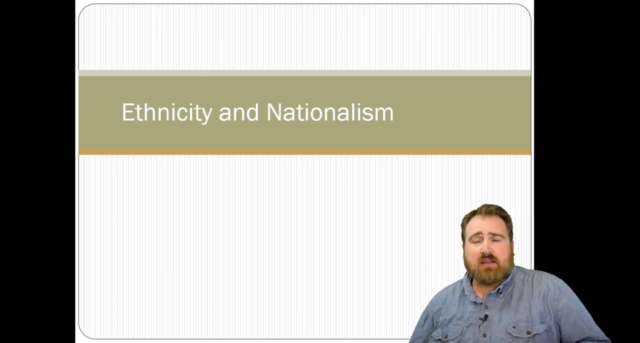 yet please do as soon as you can and and we'll go from there. okay, that's that. that's that's it for this section. we'll go on to the lecture now.